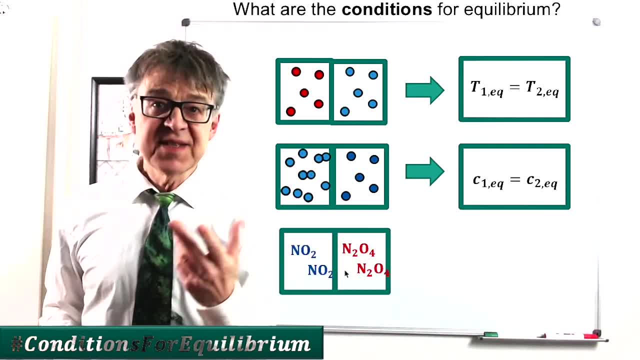 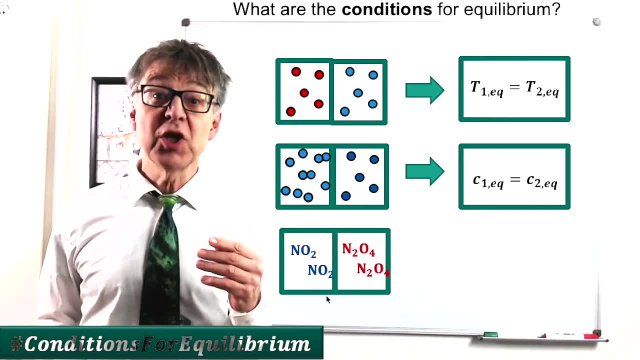 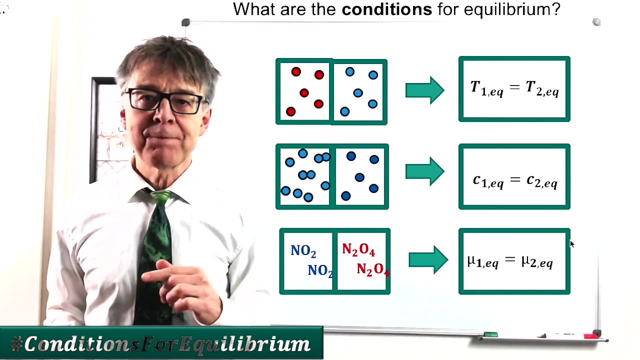 in the initial state is a measure of the distance from equilibrium. Incidentally, we can discuss chemical equilibrium in a very similar way. We have to add another equilibrium condition which states same chemical potential everywhere. More on that later. If there are temperature differences in a system, heat transfer is provoked. 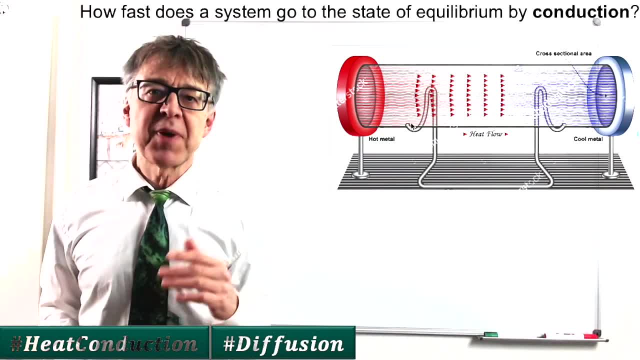 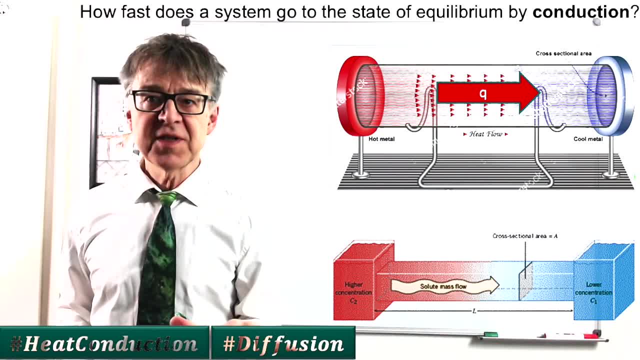 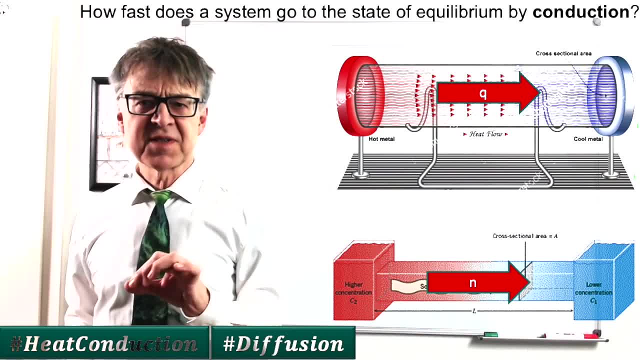 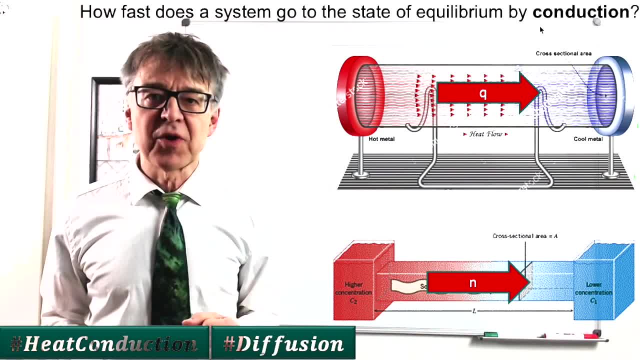 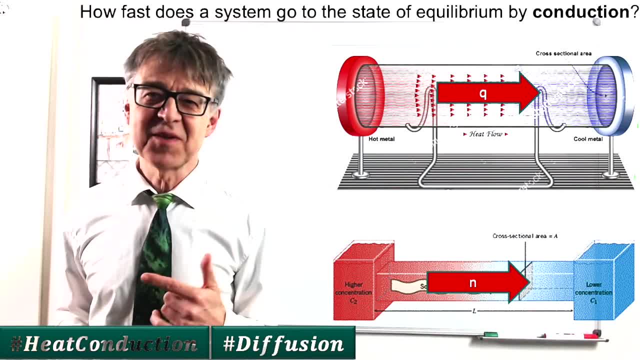 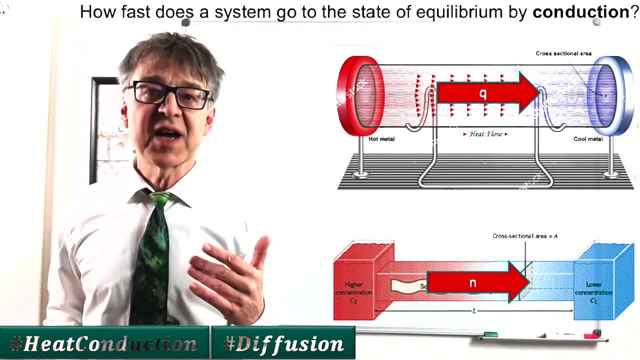 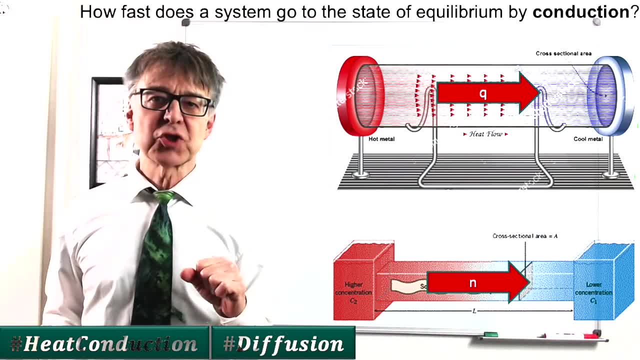 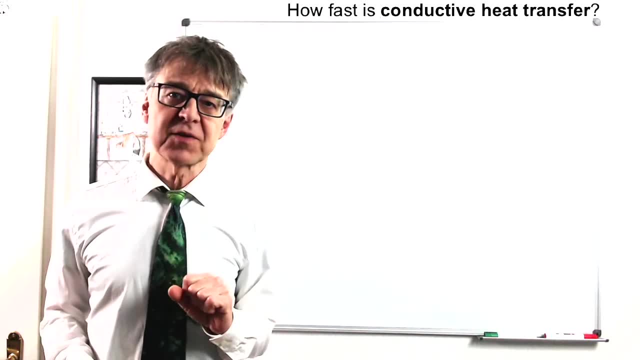 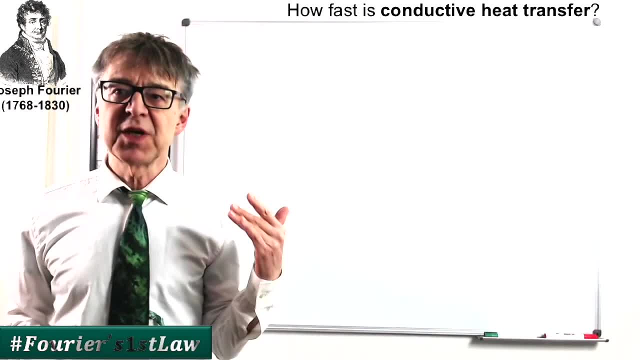 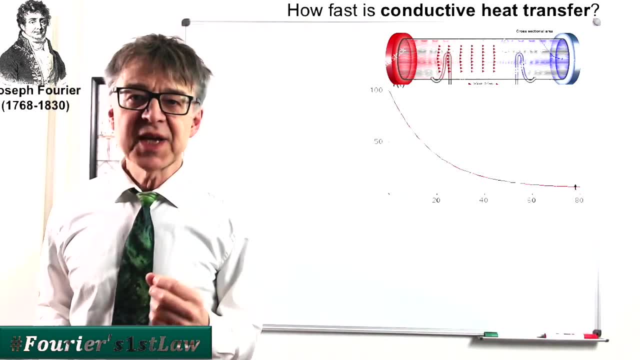 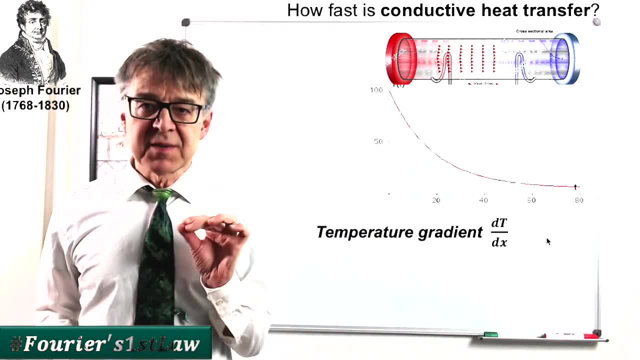 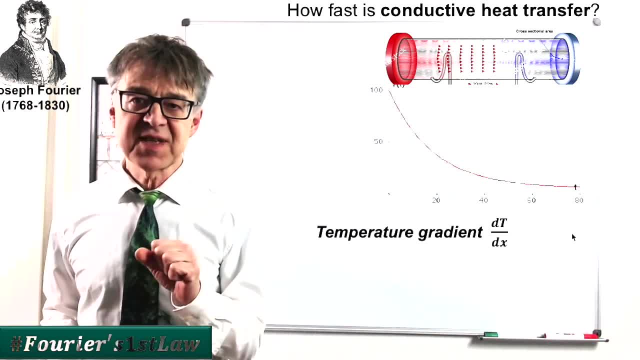 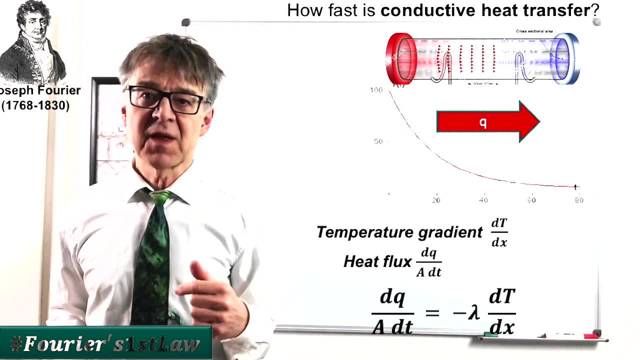 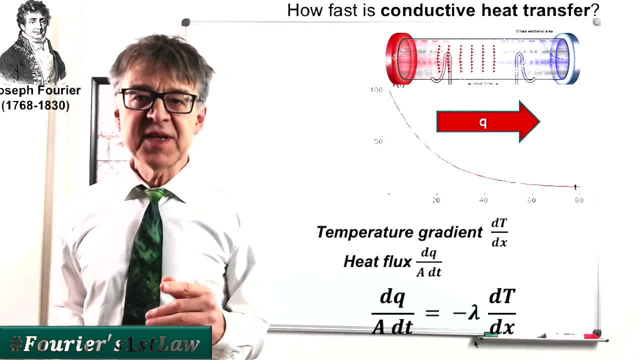 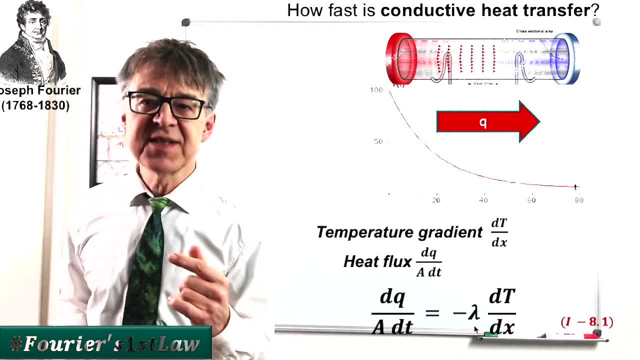 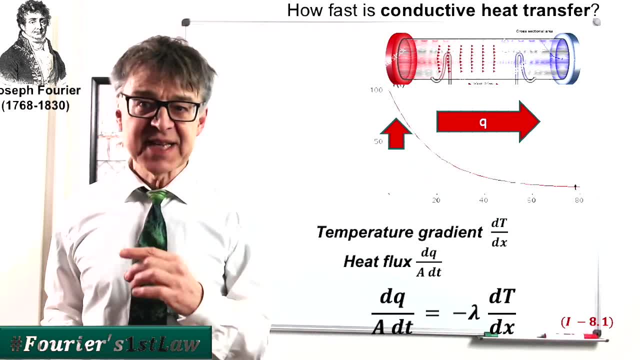 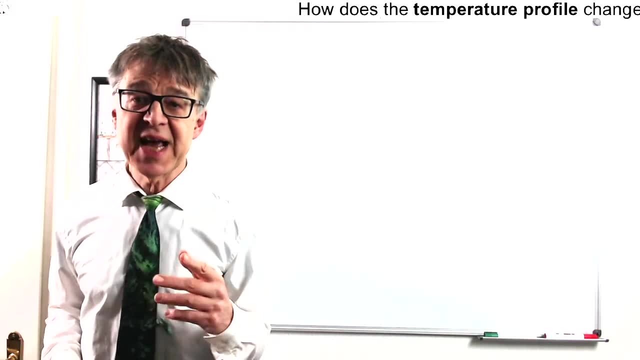 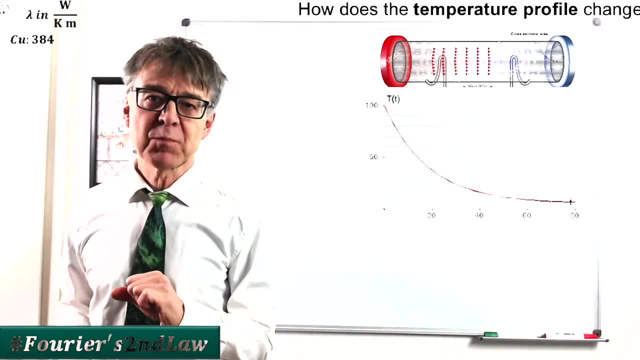 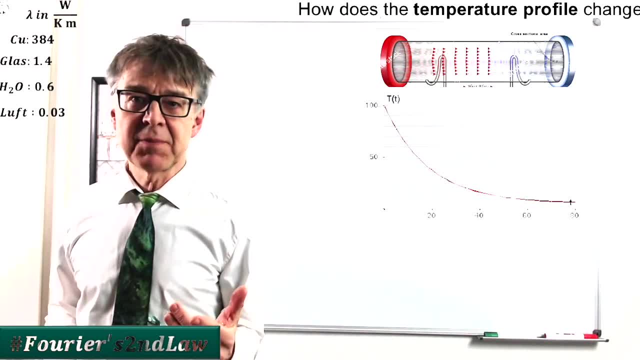 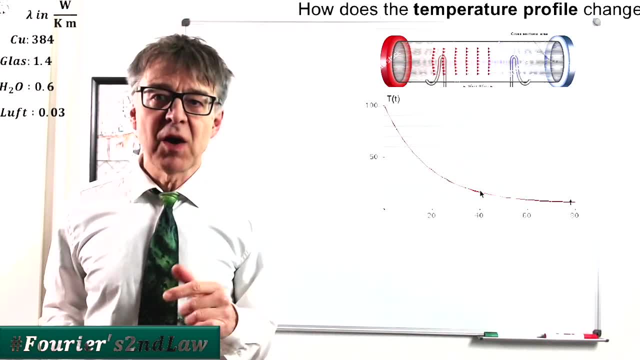 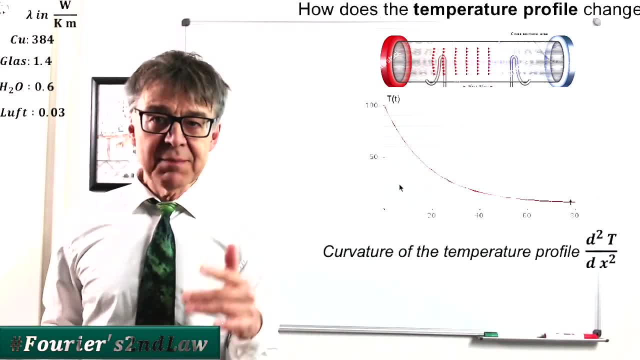 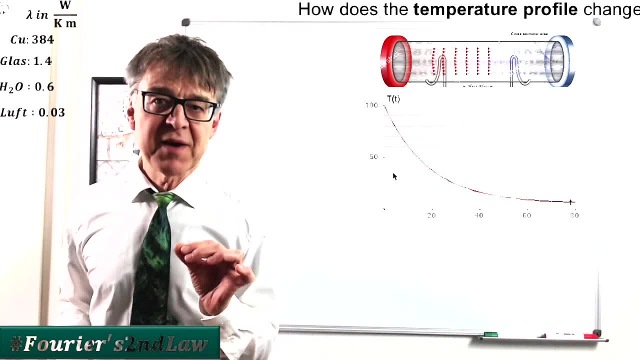 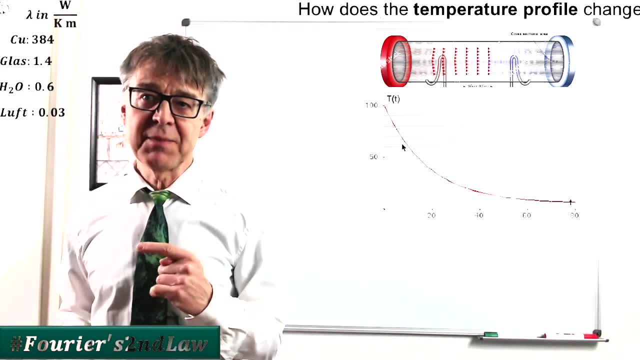 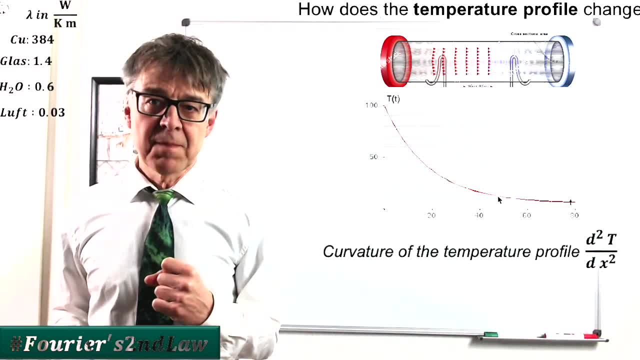 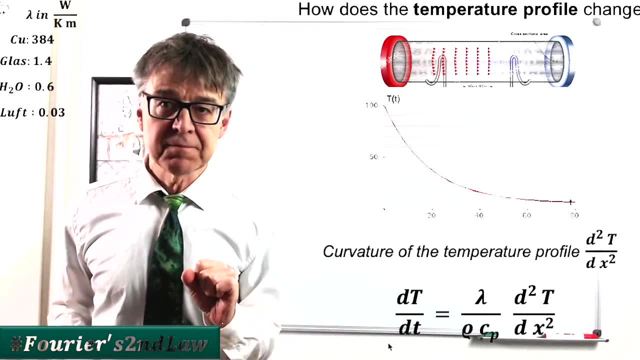 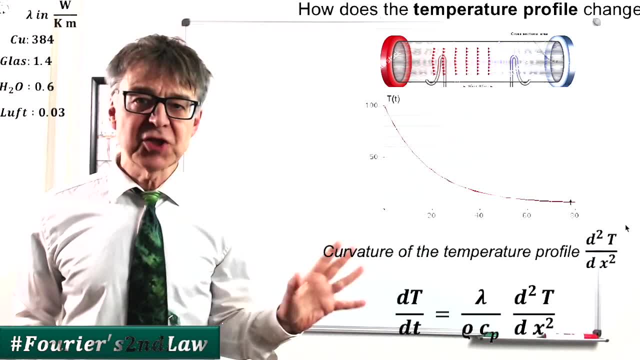 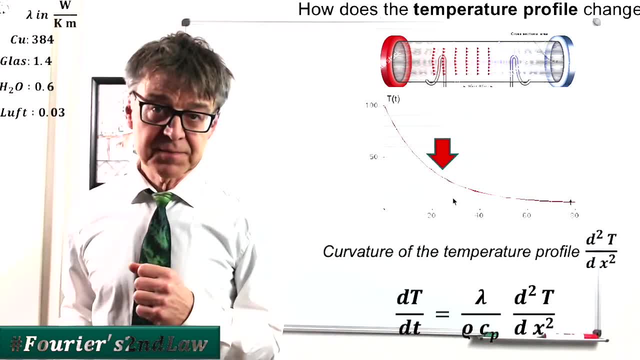 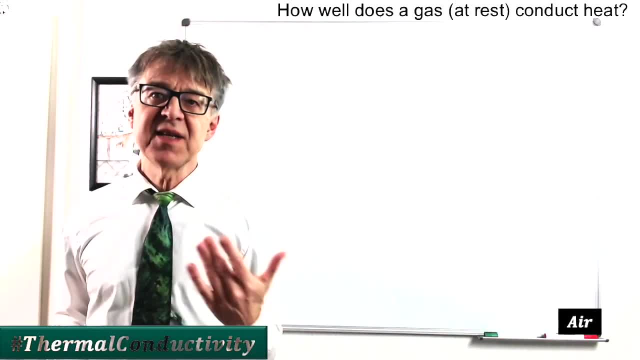 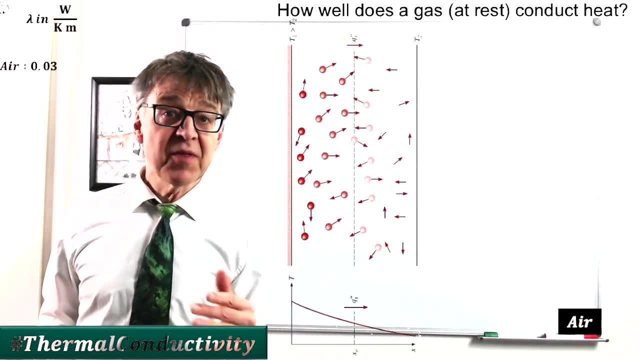 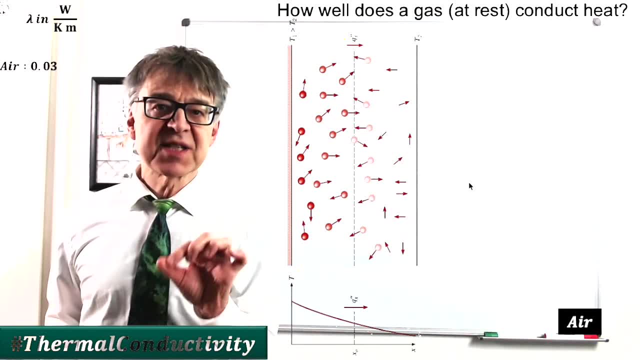 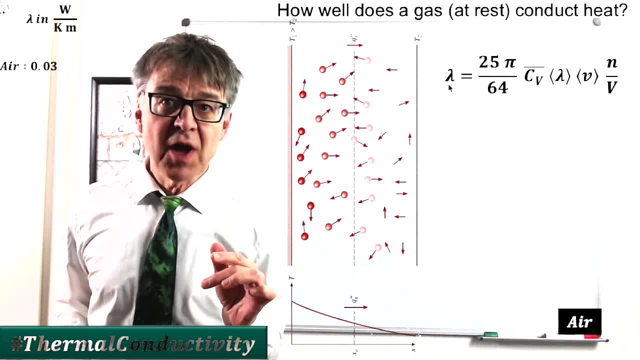 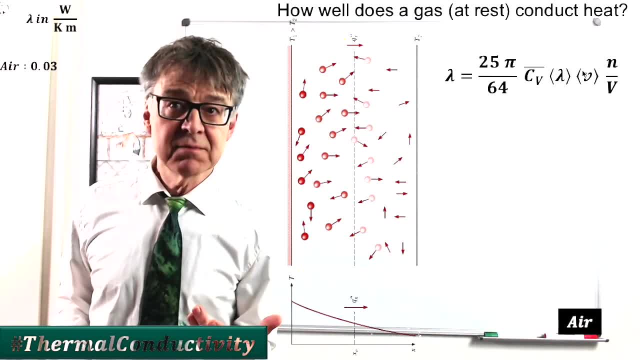 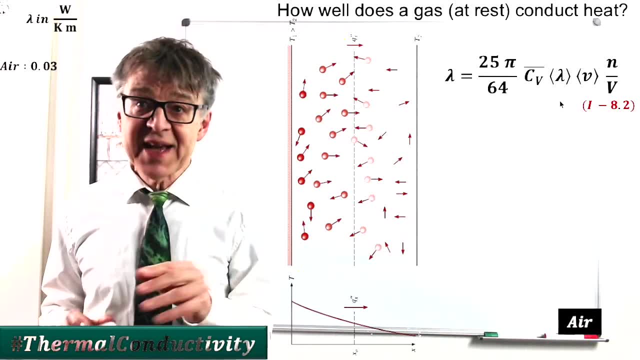 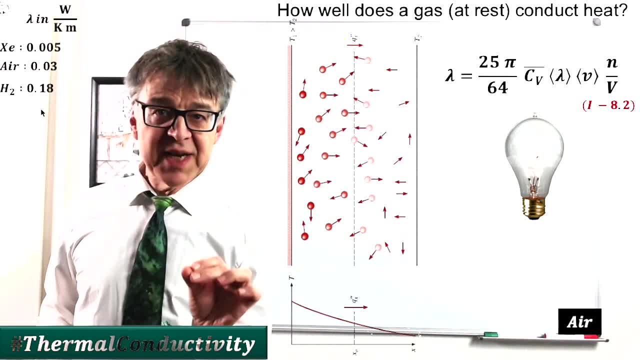 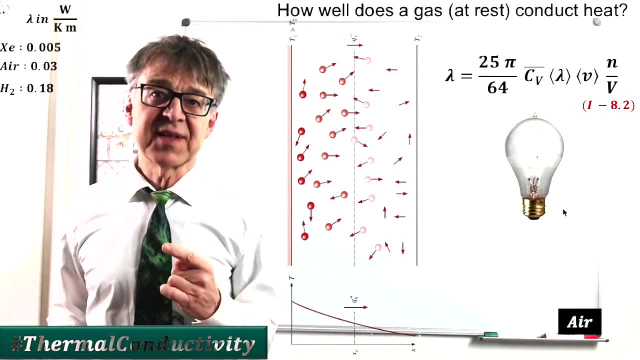 conduction occurs, which is a passive energy transfer without external forces. Heat conduction occurs, which is a passive energy transfer without external forces. Heat do have the greatest thermal conductivity in relative terms. A simple light bulb can be seen as a thermal conductivity detector. 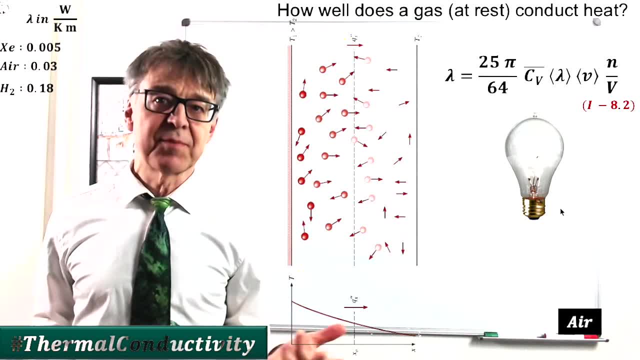 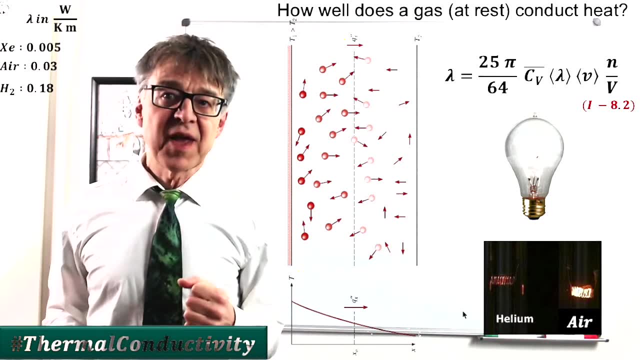 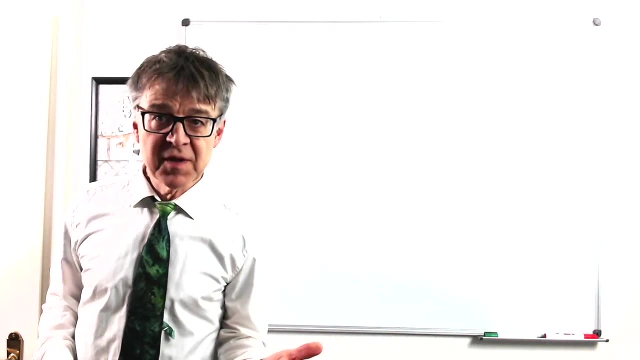 The poorer the thermal conductivity of the gas in the bulb, the brighter the filament lights up. This phenomenon is used to detect gases, for example in gas chromatographs. Diffusion is quantified by Fick's laws. These are completely analogous to Fourier's laws. 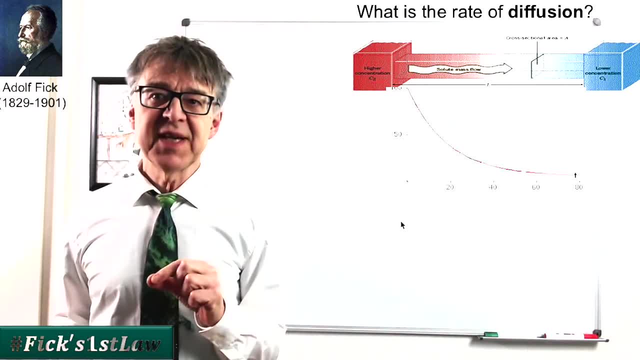 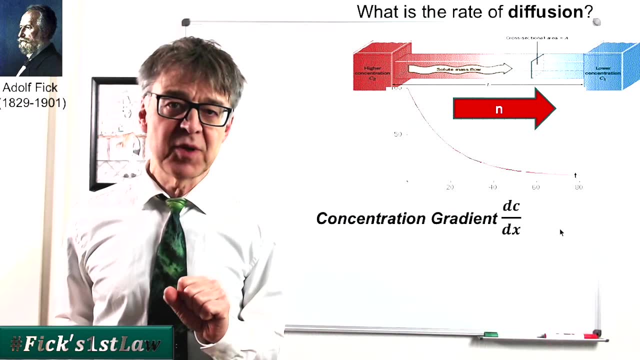 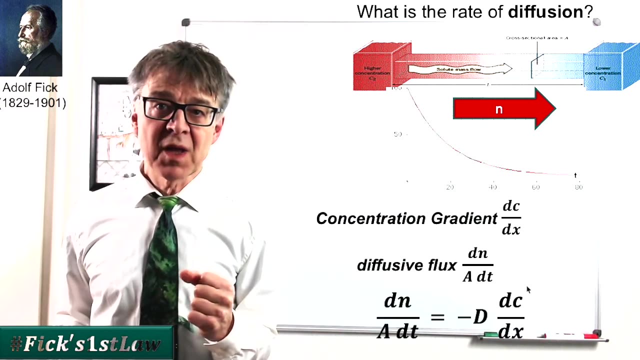 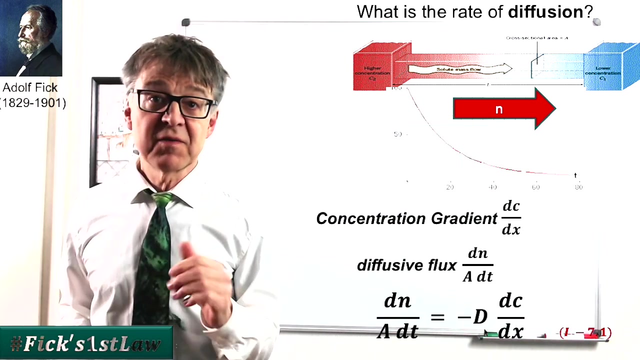 Diffusion is caused by a concentration gradient. in the one-dimensional case, dc over dx, The intensity of the passive mass transport, quantified by the mass flow density, is proportional to the concentration gradient. Where the concentration profile has the largest slope marked by the red arrow, flux is largest. 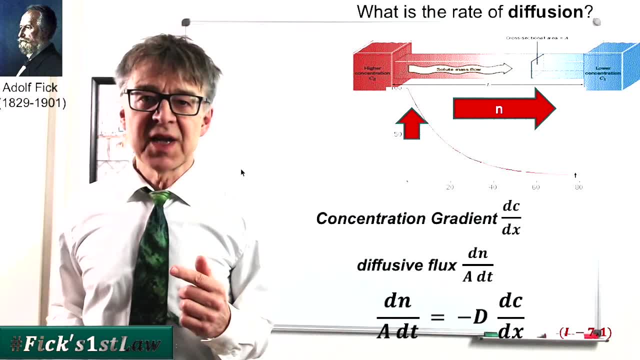 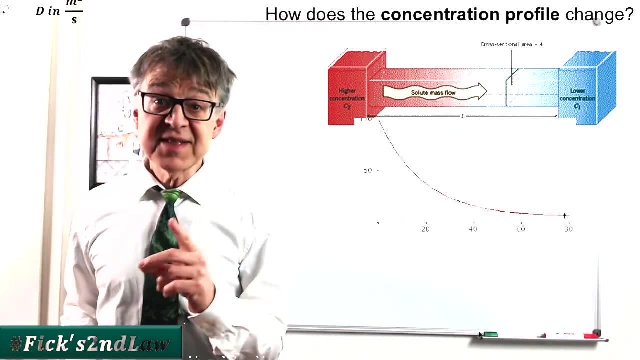 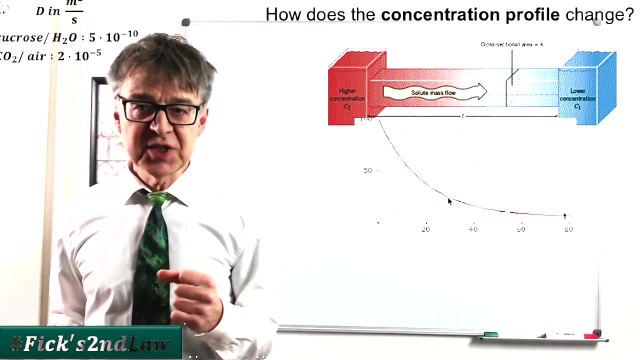 The coefficient d describes the diffusion in a medium at rest. It is much slower in a liquid than in a gas With unsteady state or transient diffusion. the concentration in the system changes over time. The change in concentration is proportional to the curvature of the profile. 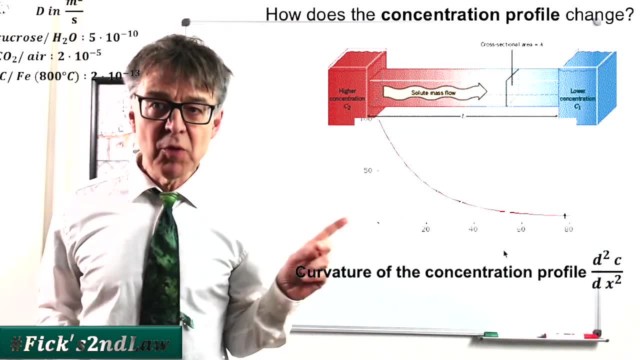 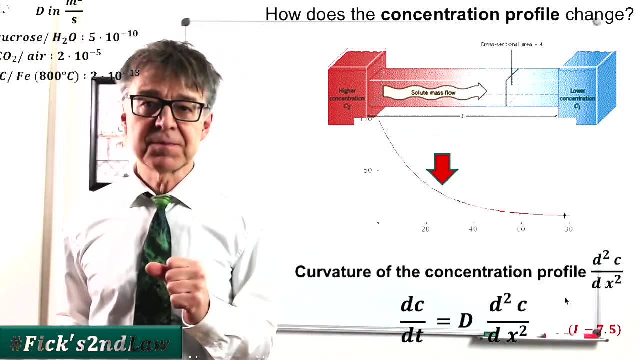 This is Fick's second law. The arrow marks the point of largest curvature in our example. At this point, the concentration will change. This is Fick's second law. At this point, the concentration will be the most. The diffusion of gases can also be explained with the kinetic gas theory. 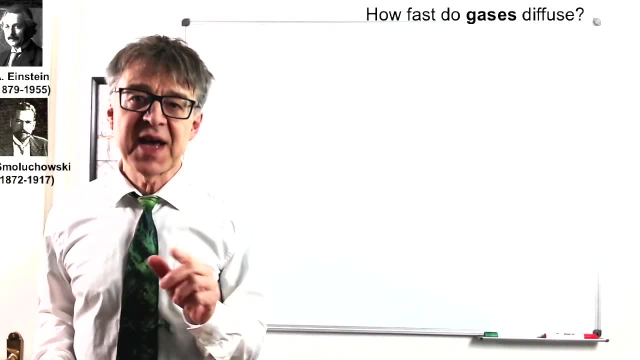 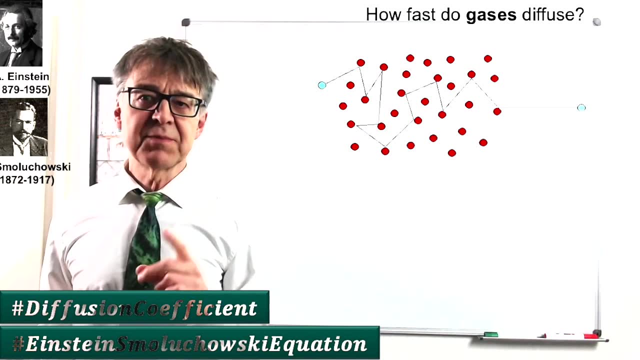 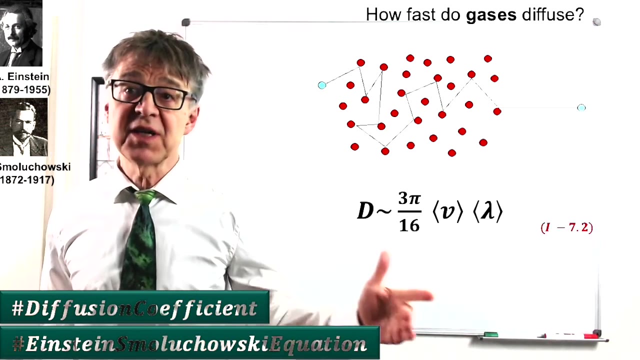 Again, small and light gases diffuse fastest. Einstein and Smolokhovski were able to explain Fick's laws with their random warp model. In particular, they were able to calculate the displacement x. This is the distance to quantify how far a particle moves from its starting point by diffusion. 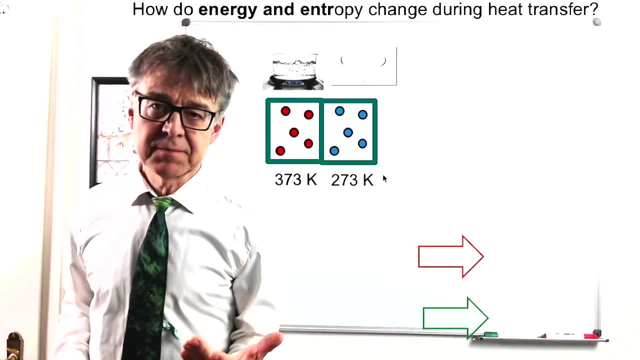 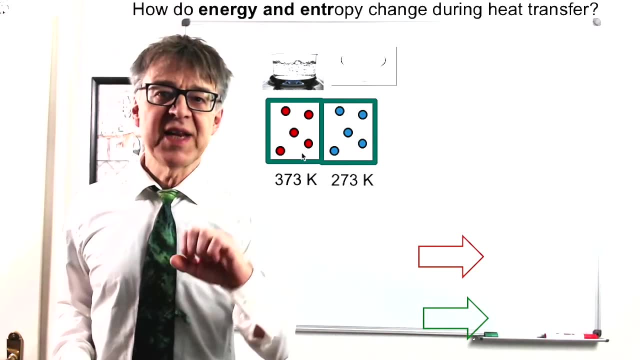 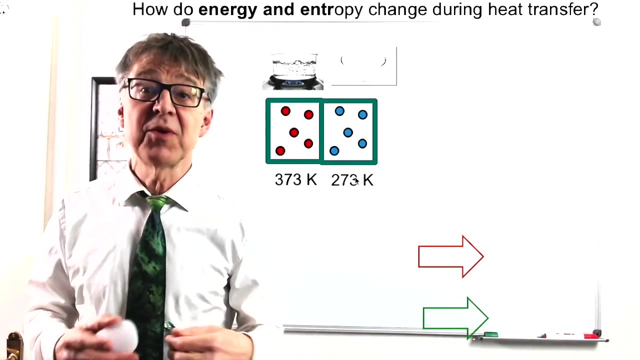 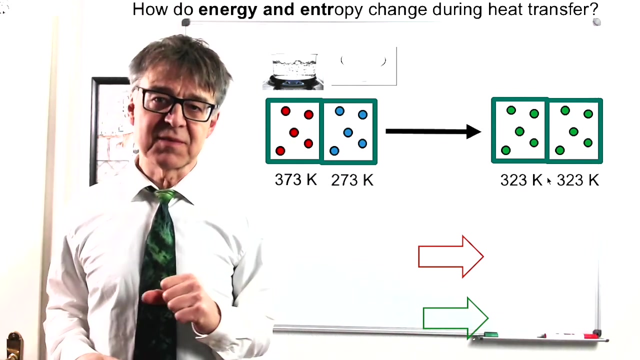 Let's discuss a heat transfer experiment thermodynamically. Consider two subsystems: One liter of water at 100°C and one liter of water at 0°C. After bringing these systems in thermal conduct, eventually thermal equilibrium will be reached with a uniform temperature of 50°C in both of the systems. 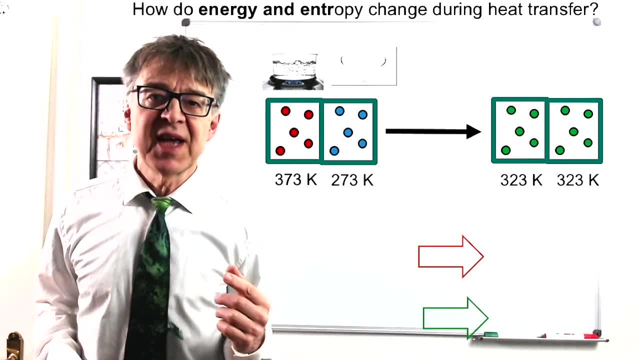 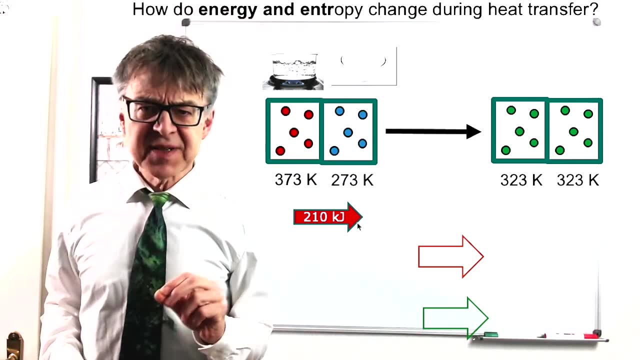 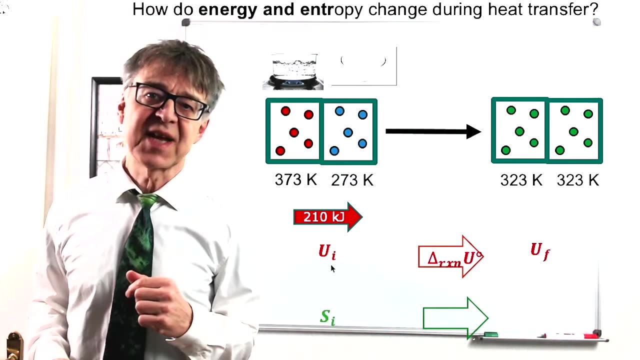 Using the heat capacity of water, we may easily calculate the transferred heat to be 210 kJ. Let's look at this process like a thermodynamicist and discuss it in terms of energy and entropy using the first and the second law. The letter U stands for internal energy. 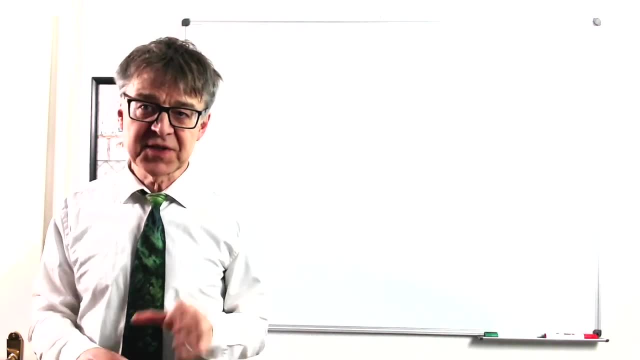 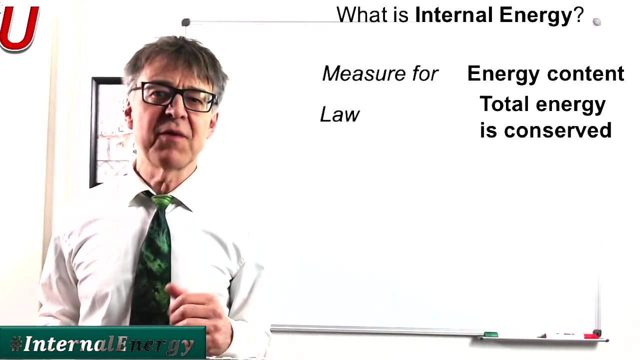 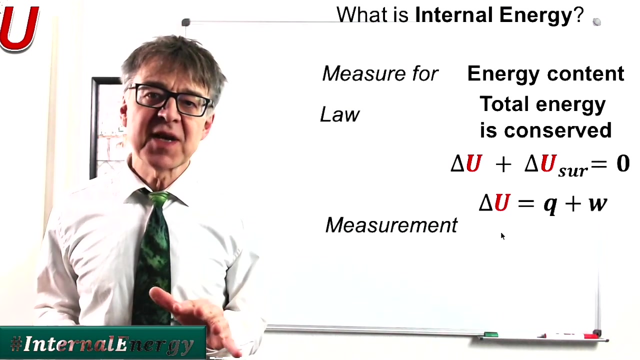 This is a measure of how much energy is inside of a system. The definition of this quantity makes sense because the first law states that the total internal energy of the universe remains constant. We can measure internal energy change of a system by simply adding heat and work. 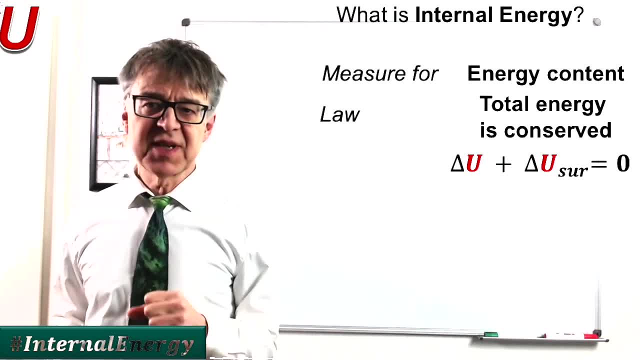 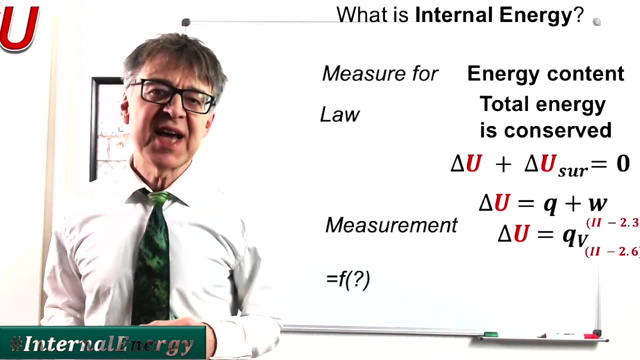 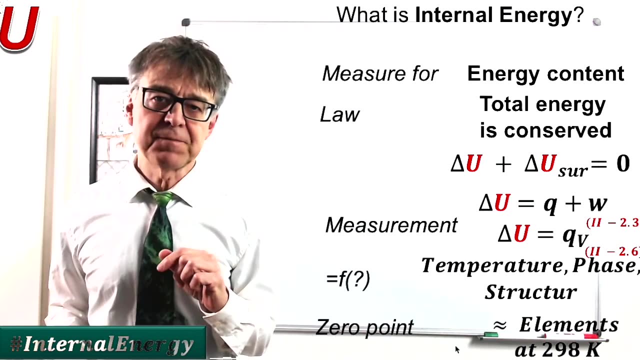 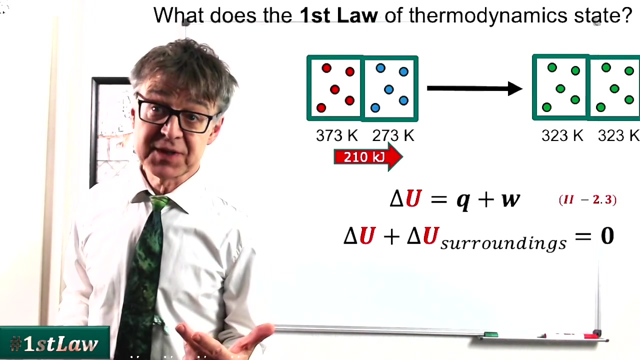 which accompany the process. In every process in which heat or work are involved, the internal energy changes. The elements at 25°C were arbitrarily chosen as the zero level for energy. Let's discuss the thermal equilibrium experiment thermodynamically, in energy terms. 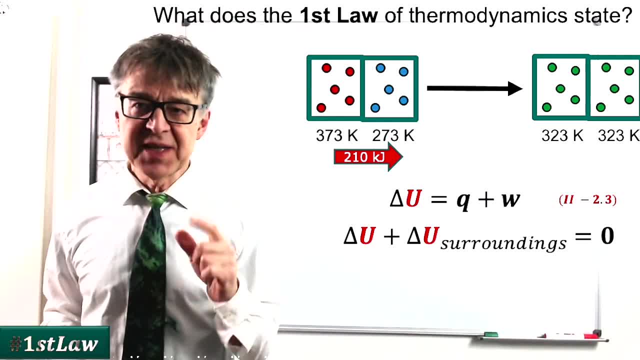 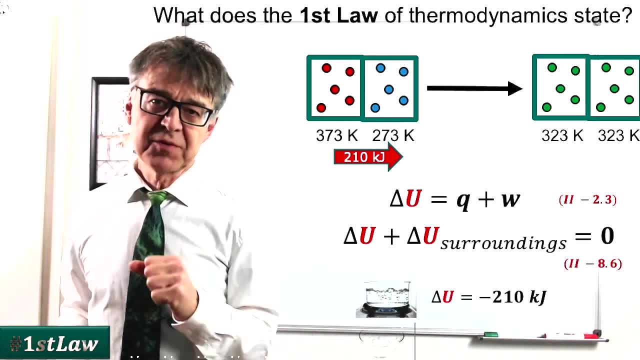 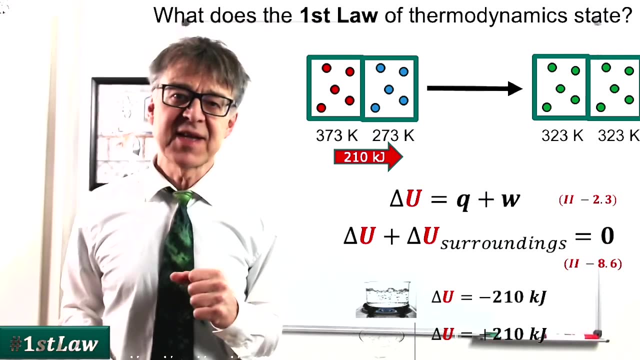 looking through energy glasses, so to speak, and apply the first law. The originally hot water has lowered its internal energy by 210 kJ. The originally cold water increased its internal energy by exactly the same amount, 210 kJ. The letter S stands for energy. 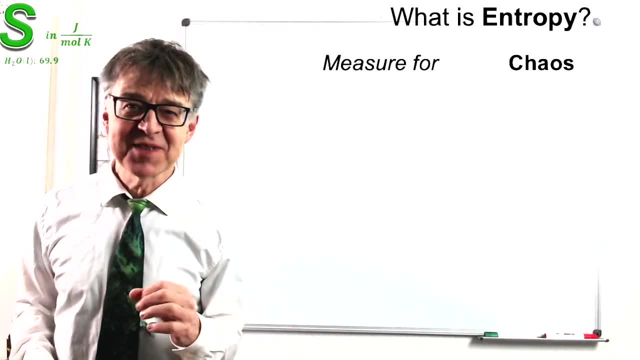 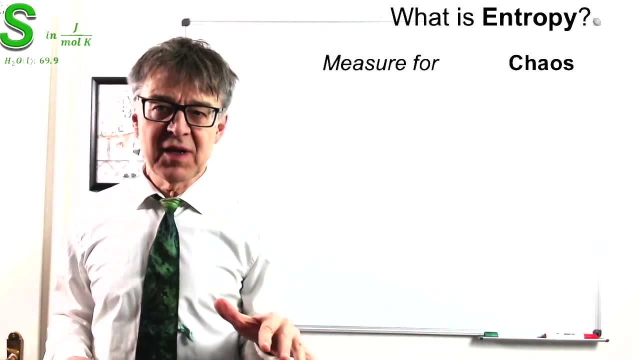 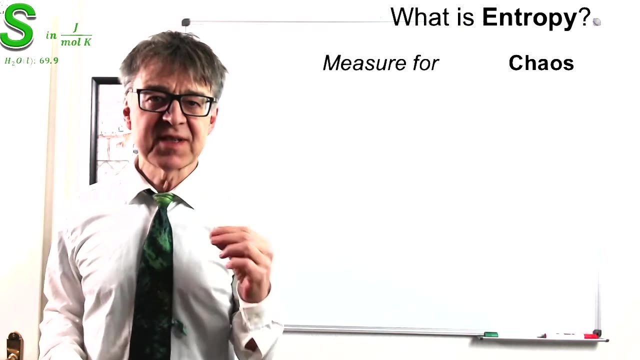 And entropy. Entropy is, in layman's terms, a measure of the disorder or chaos in a system, a measure of energy dispersal, of how spread out the energy is. The introduction of this state function makes sense because the second law simply states: 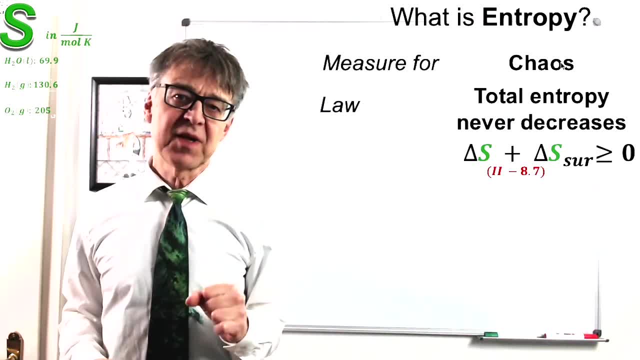 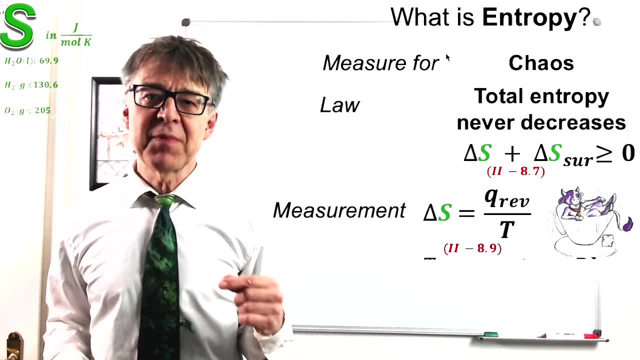 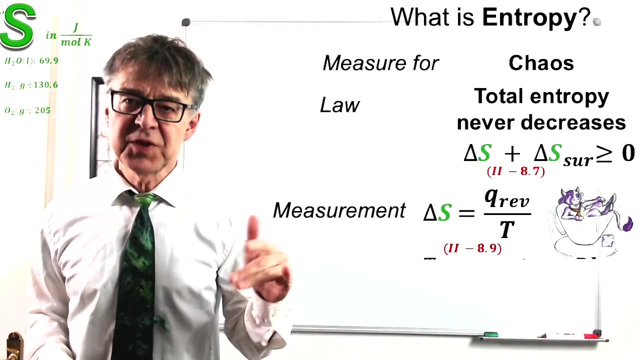 that the total entropy of the universe can only increase. According to Clausius, the change in entropy of a system can be measured by the so-called reduced heat Q divided by T QT. This little QT may serve as a mnemonic for this definition. 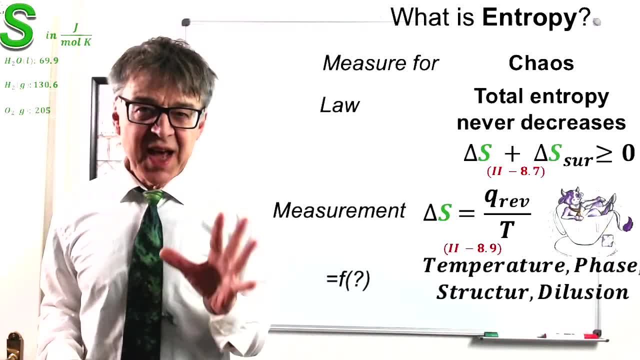 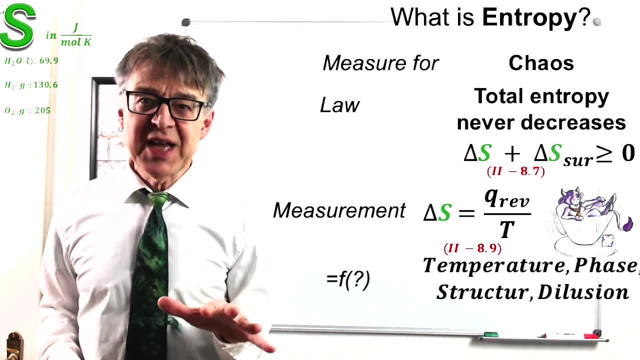 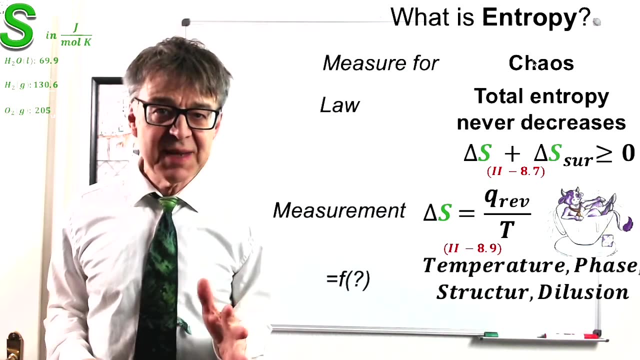 and help you to remember Clausius' equation. Entropy shows similar dependencies as internal energy, but, unlike energy, entropy also depends strongly on dilution. The temperature of an ideal gas at room temperature has the same energy whether it's at one bar or at two bars pressure. 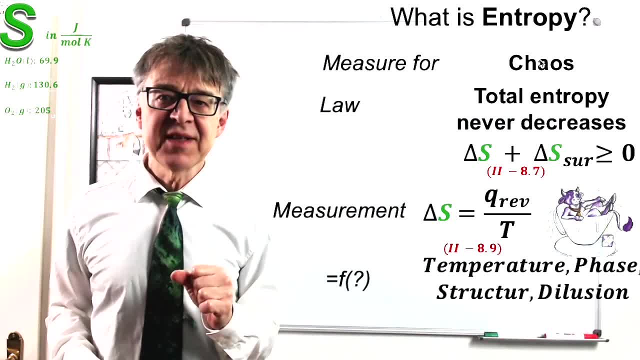 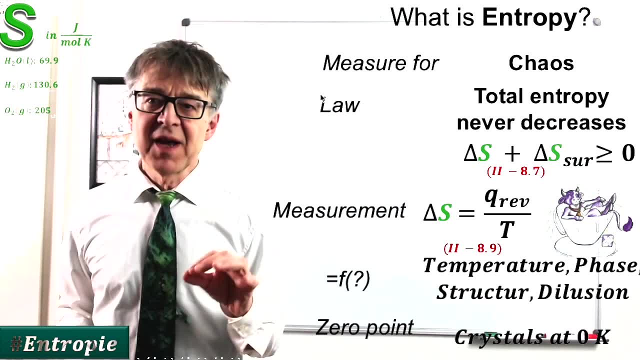 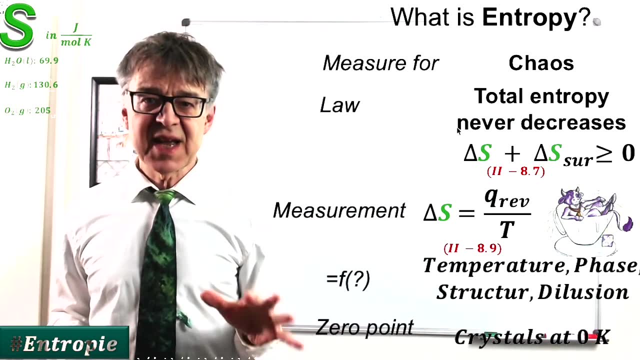 However, the one-bar gas has a higher dilution and thus the higher entropy. The zero point of entropy is not arbitrary, but given by nature. The third law of thermodynamics states that in ideal crystals at zero Kelvin, we will have an entropy of zero. 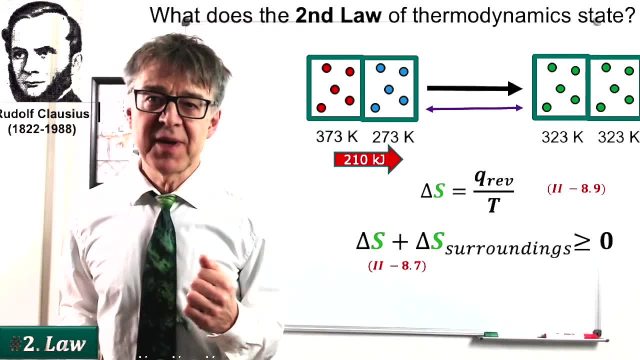 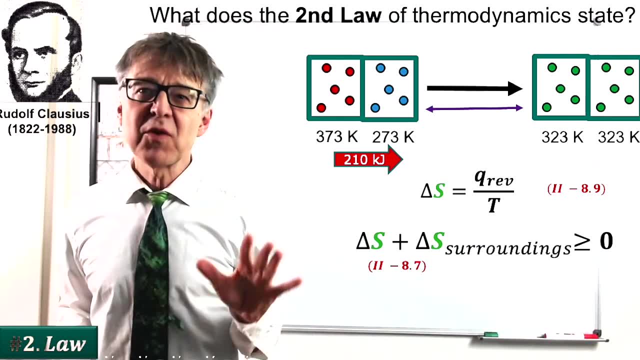 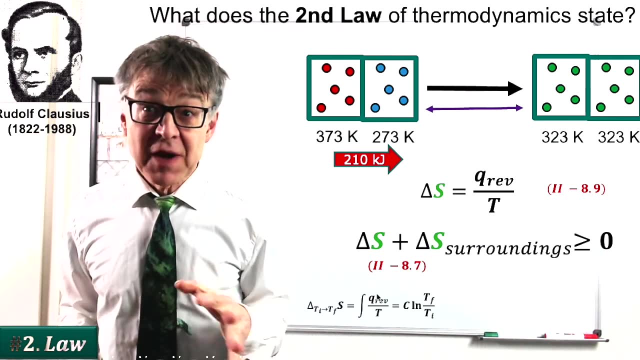 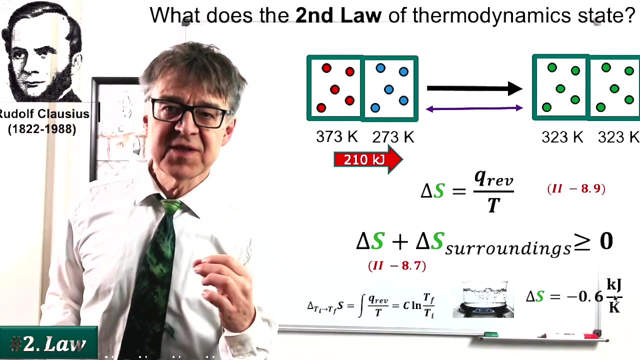 Now let's discuss the thermal equilibrium experiment in terms of entropy. Let's put on our entropy glasses. The entropy of the originally hot water has decreased. We use our QT-Clausius equation. We have to integrate, because the temperature is not constant, and get an entropy decrease of negative point, six kilojoules per Kelvin. 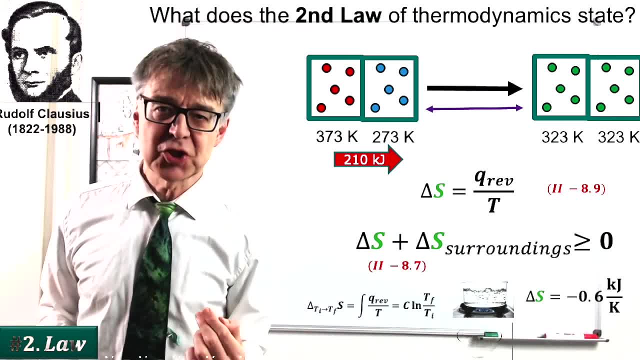 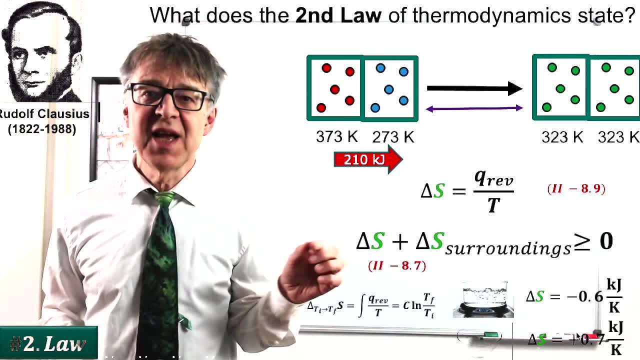 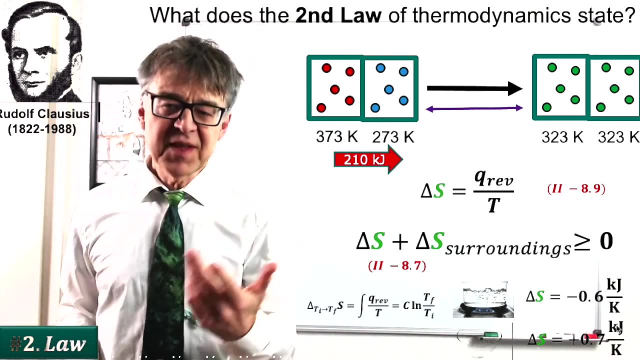 Using the same equation and plugging in the temperature, the temperature changes for the other subsystem, We calculate that the entropy of the originally cold water has increased, but by a larger amount. Our overall entropy was just generated in the process. This holds for every process in the universe which is spontaneous. 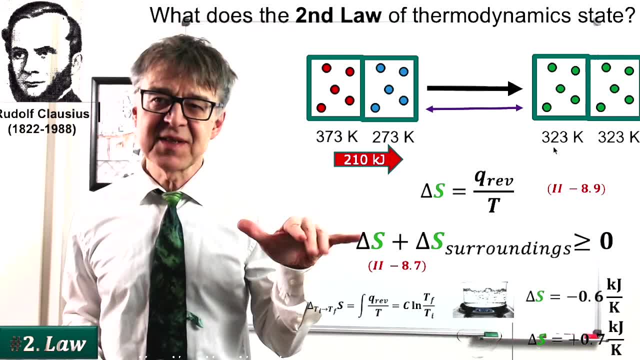 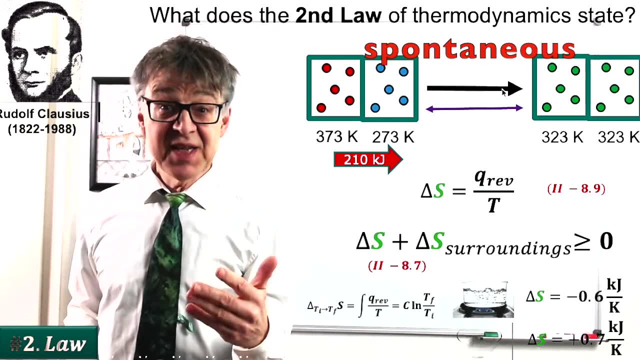 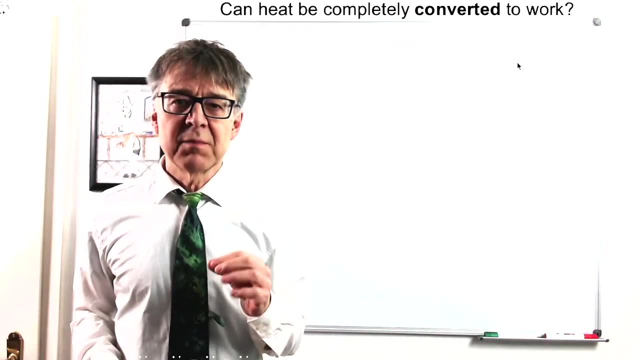 Processes in which the total entropy increases are called irreversible. They can only take place in one direction. Spontaneous heat transfer from hot to cold is irreversible, as just described. Mr Carnot had thought about how to gain work from this process. 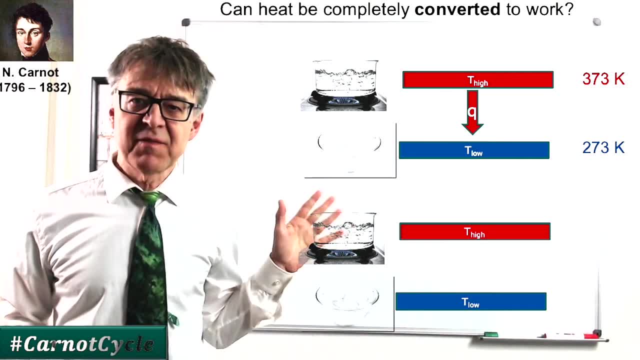 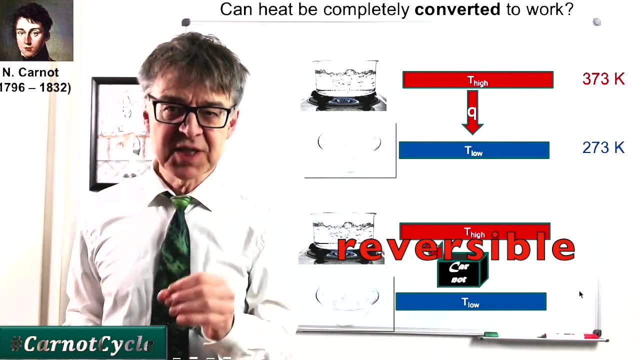 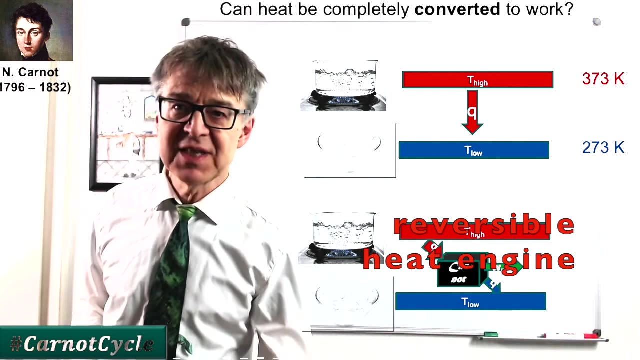 He has described a machine that makes this very process- heat transfer from hot to cold- reversible and thus derives the maximum possible amount of work from it. The Carnot machine is therefore a heat engine like a steam engine or a diesel engine. 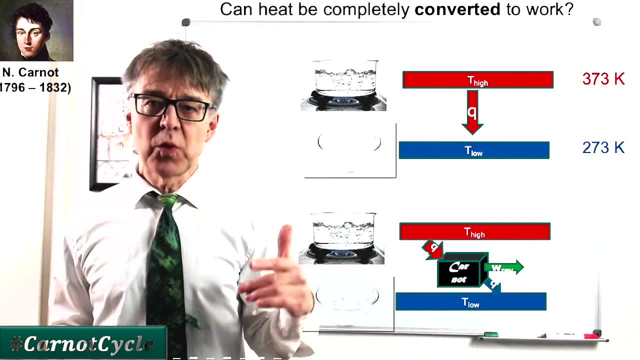 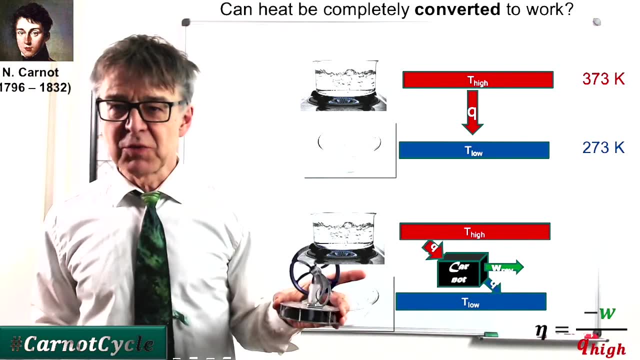 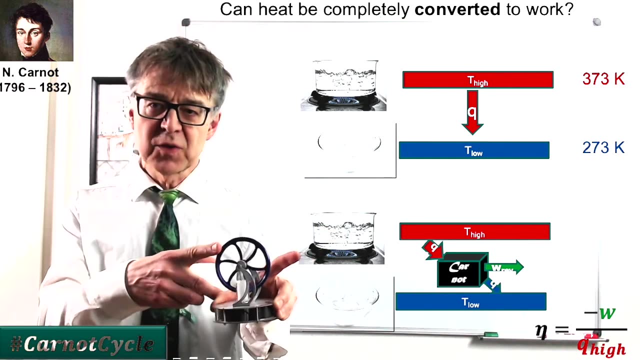 or like a Stirling engine, It converts heat into work with the best possible efficiency. eta A Stirling engine is also a heat engine. We have two temperature levels between which heat is transferred and which is converted into work to a certain fraction. 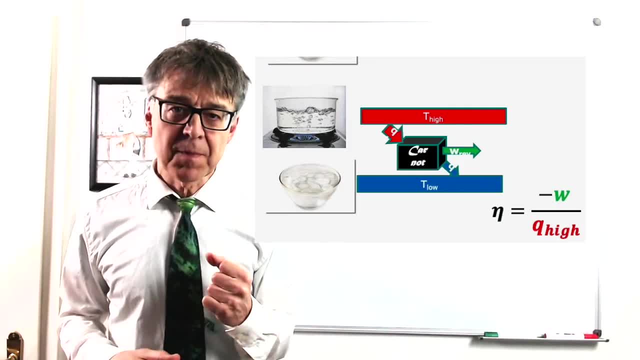 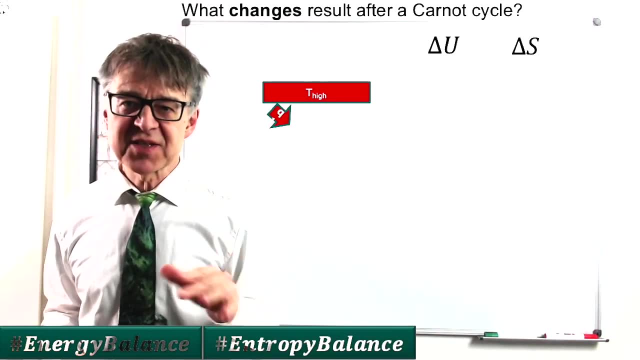 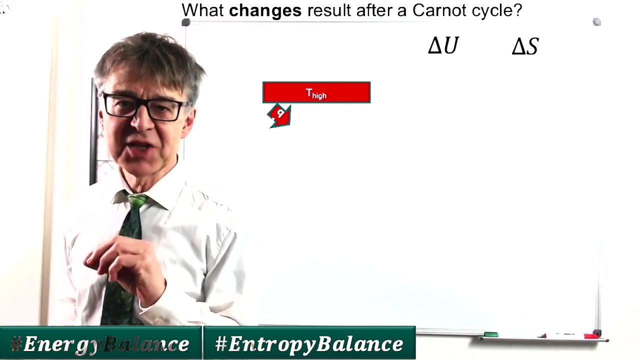 We now consider a working cycle of a Carnot machine. We are talking through our energy and entropy classes. Let's examine the various subsystems step by step in terms of their energy and entropy change. When the Carnot machine is running, both the internal energy and the entropy of the upper temperature level decrease. 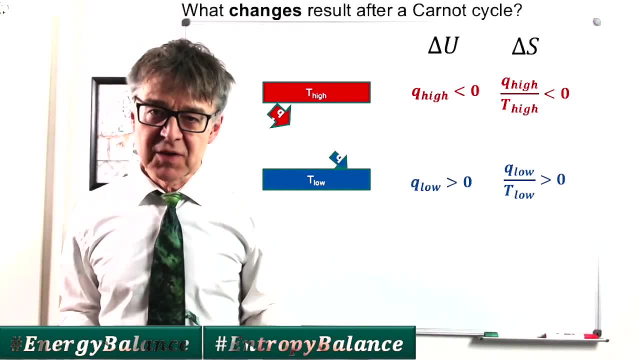 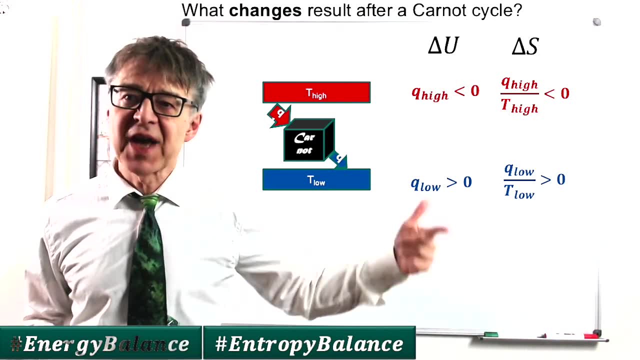 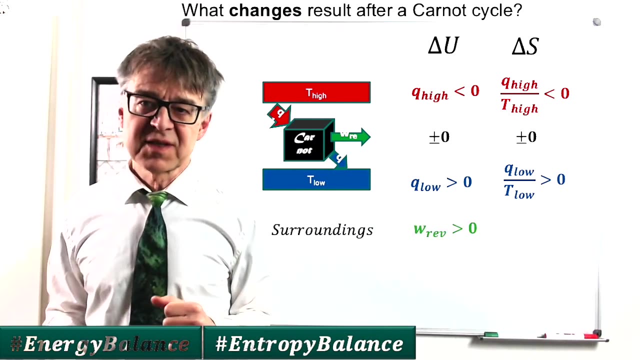 The reverse applies to the lower temperature level: The internal energy increases and also the entropy increases. The Carnot machine itself goes through a cycle, So it changes neither energy nor entropy. The surroundings gain work, so they increase their internal energy. However, the entropy of the surroundings remains constant. 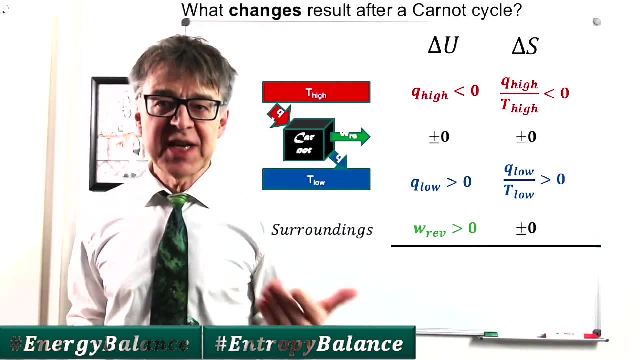 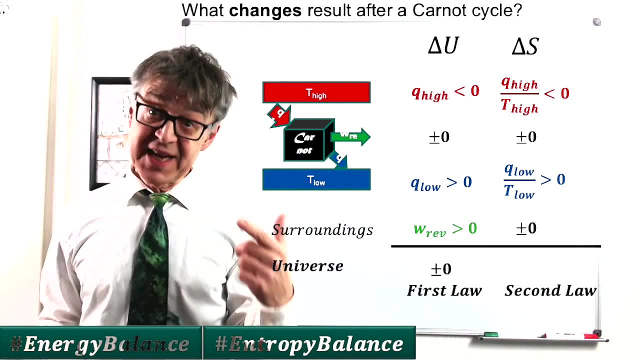 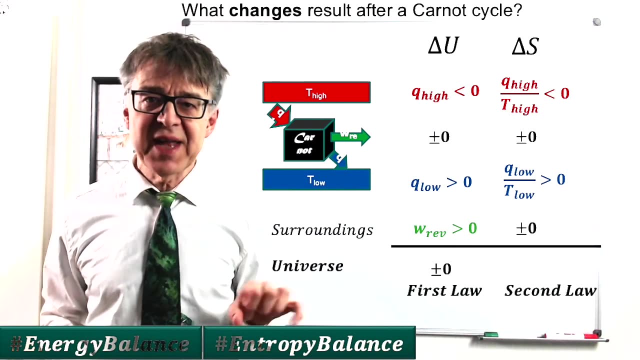 According to the first law, the exchanged energies must add up to zero. Energy can neither be generated nor destroyed. According to the second law, entropy can never decrease. That means the sum of the entropy amounts must be greater than or equal to zero. 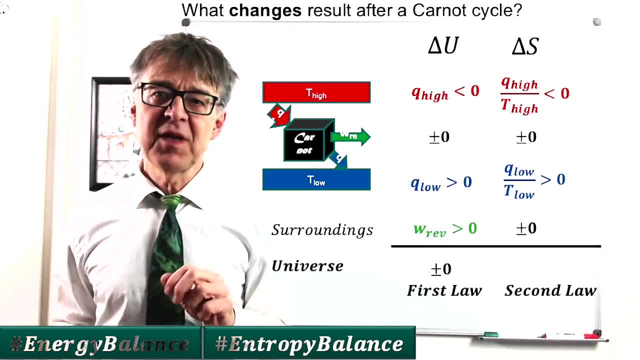 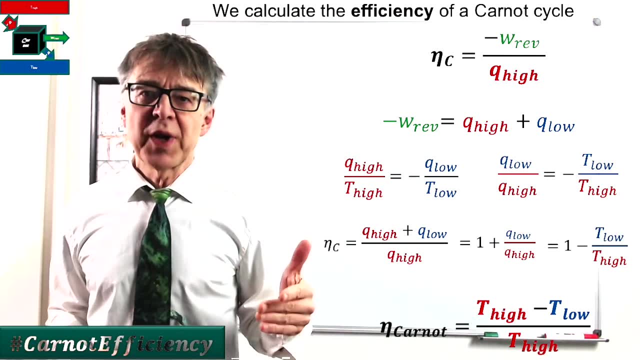 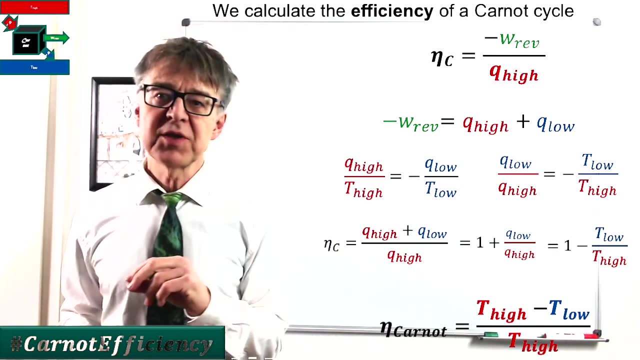 The Carnot machine works ideally reversible, which means that the total entropy change is zero. By combining these two equations we get the Carnot efficiency eta to delta T over T sub pi. This is one of the most important equations in thermodynamics. 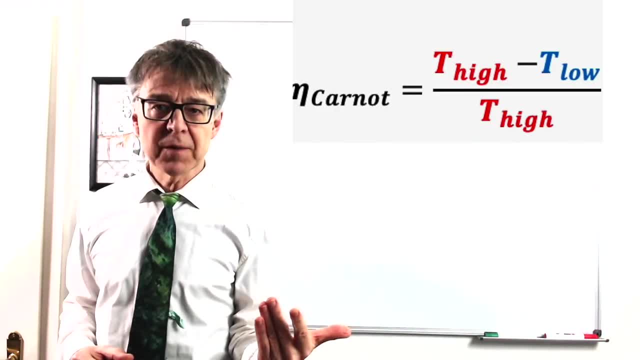 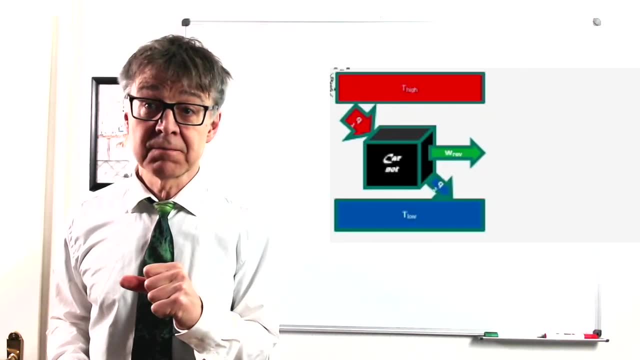 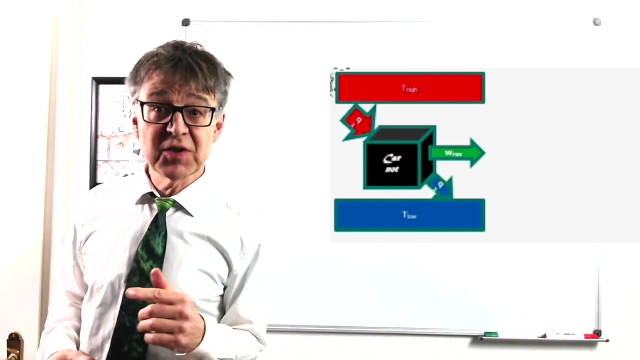 It limits the conversion of heat into work. The temperature difference between the temperature levels of a heat engine determines the efficiency. A heat engine with the two temperature levels 0°C and 100°C therefore has an efficiency of approximately 25% 100% heat from the high temperature level. 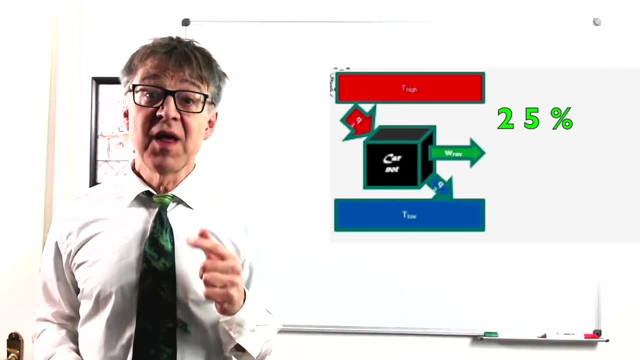 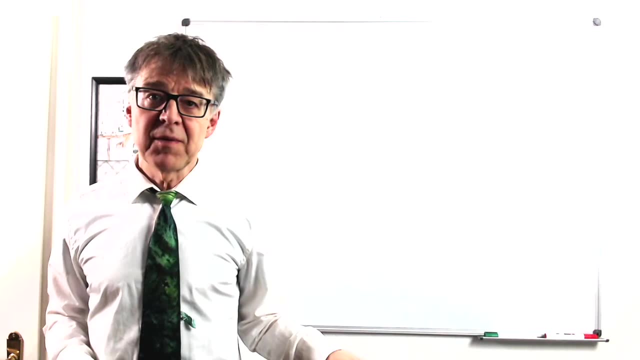 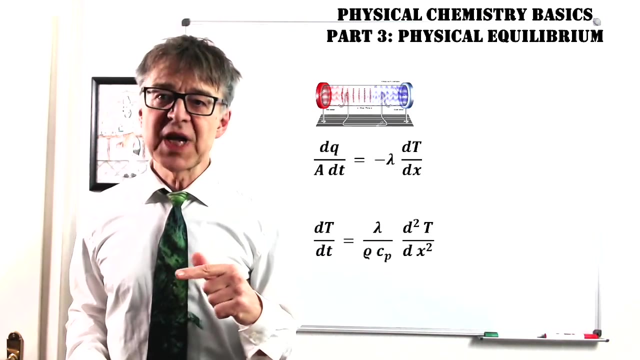 is only converted to 25% of work. The remaining 75% heat flows as waste heat into the low temperature level. Let's summarize: The conductive transport processes of thermal conductivity and diffusion can be described by similar laws. These are Fourier's laws and Fick's laws. 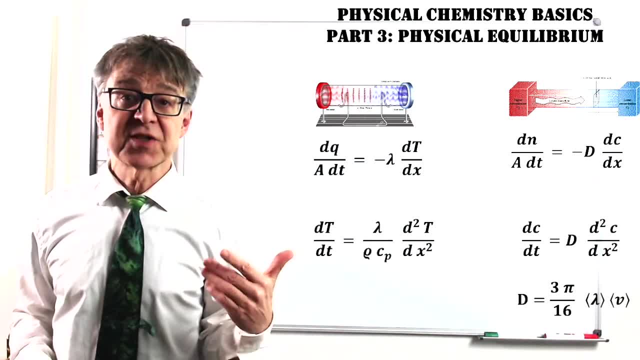 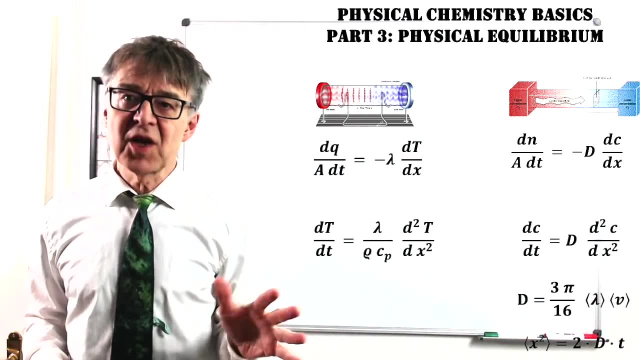 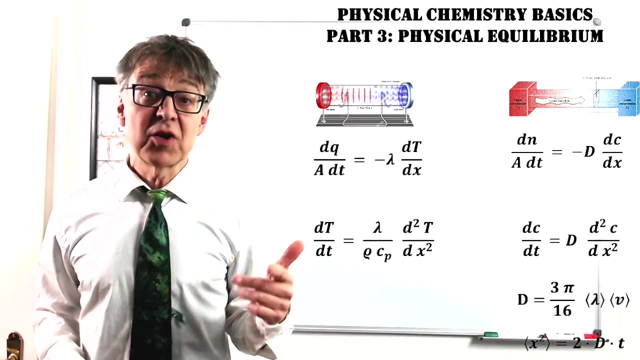 Small and light gas particles show both the largest heat conductivity and diffusion coefficient. While the complete conversion of work into heat is not a problem, the conversion of heat into work is only possible with a certain efficiency. According to Carnot, this efficiency cannot exceed: 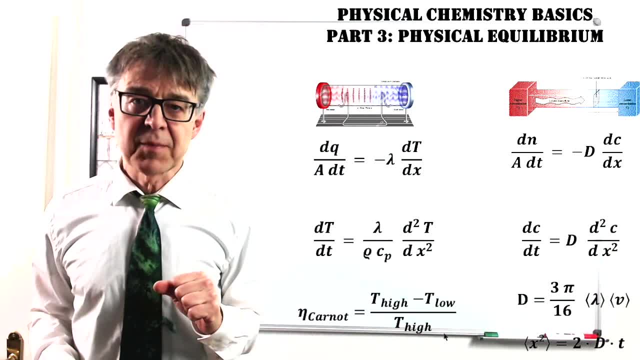 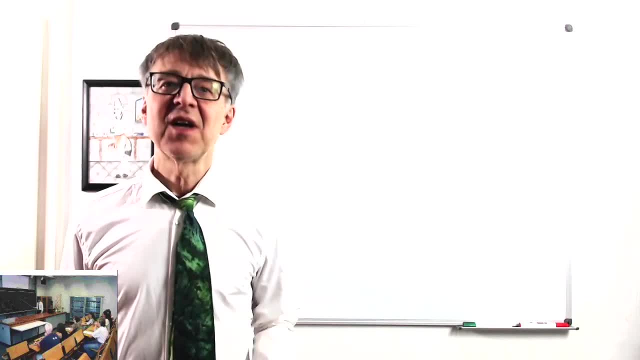 delta T over T sub pi. More information about the topic you'll find in the book and in the lecture. Thanks for watching. 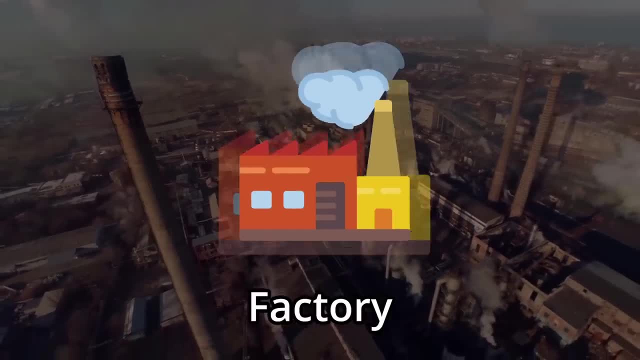 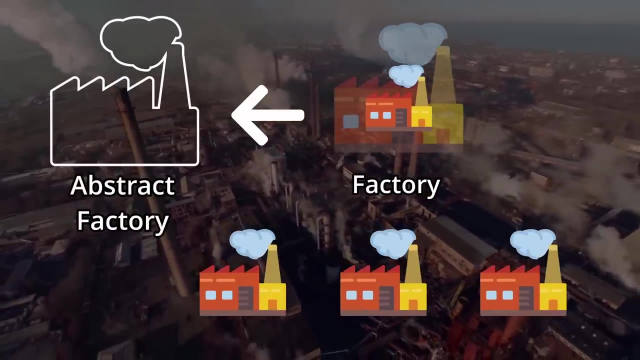 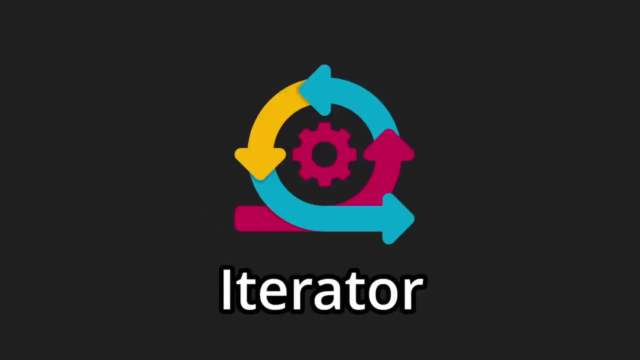 I heard you liked factories, so I made you a factory inside a factory which inherits from an abstract factory, so it can create new factories. But enough about programming in Java. In this video we will learn about 8 design patterns every developer should know. 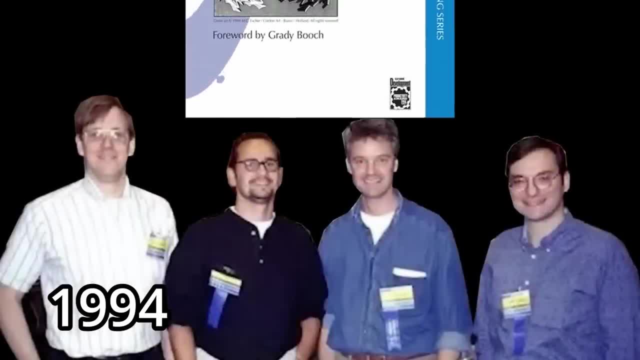 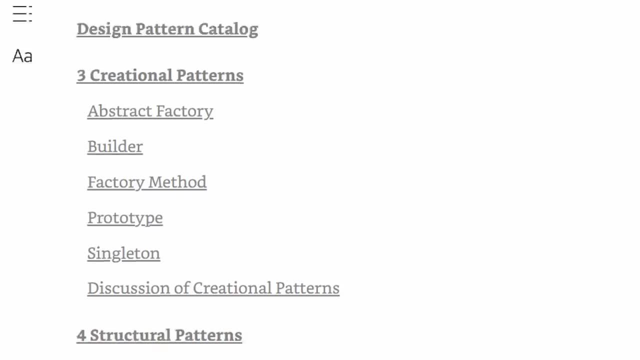 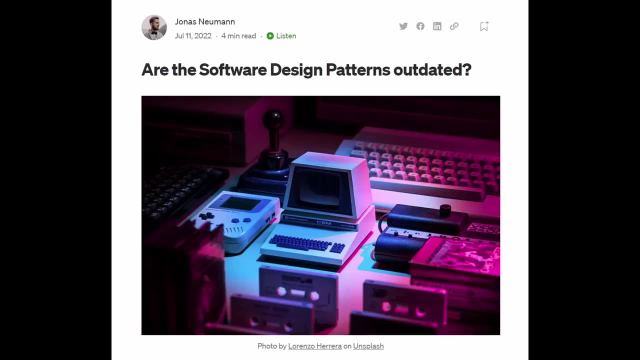 In 1994, the Gang of Four released the holy book Design Patterns, introducing 23 object-oriented design patterns falling into one of three buckets: Creational patterns, structural patterns and behavioral patterns. While some argue that it's dated, the fact that a 30 year old book is still being discussed-